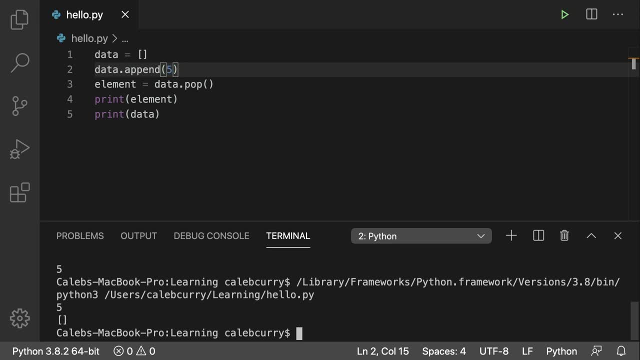 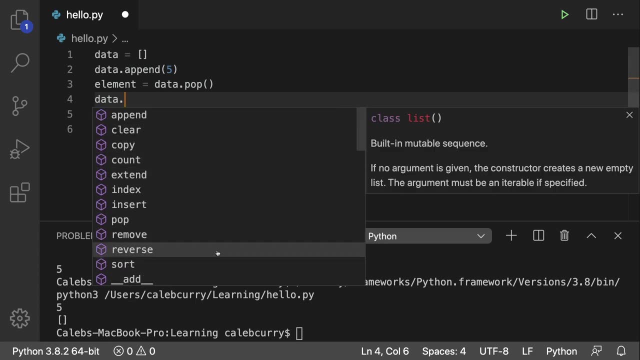 as a stack. Yes, lists have other operations, So, for example, we can go data dot and pretty much anything in this list is available to us for use. However, we, probably for best practices, want to limit to just a few of these: probably pop and probably append. Now you might be wondering: why would you use a list and 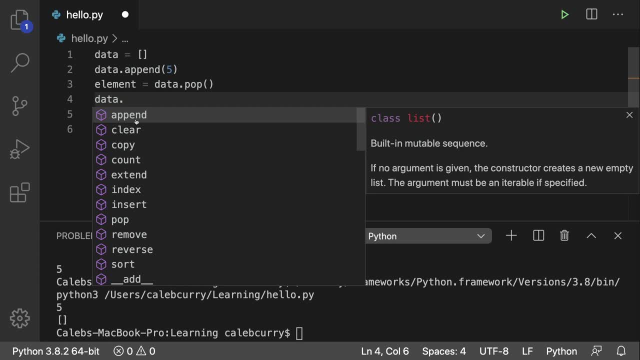 then pretty much limit its functionality by only using a few of the methods available to us. Well, it's basically for our sake. If we are trusting a stack to work a certain way, then we want to abide by the rules of a stack, If we're. 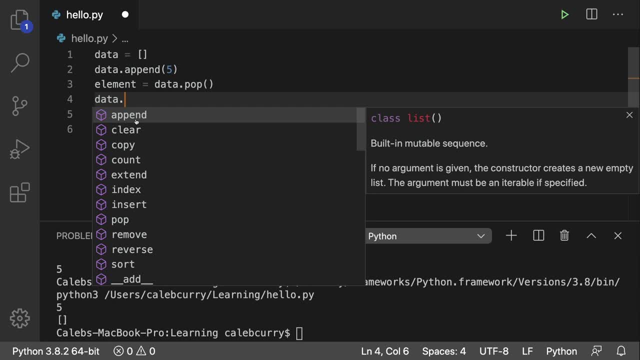 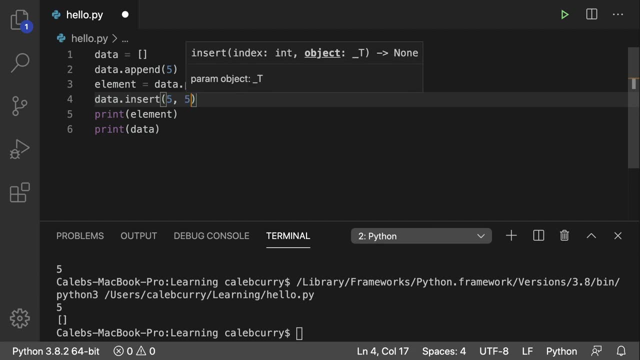 expecting a stack to only allow us to put things on top of the stack and remove things from the top of the stack. but then I go in here and say: insert and pass in some index and put some data in here. Well, that's just going to totally throw the integrity of our stack into question. So it's 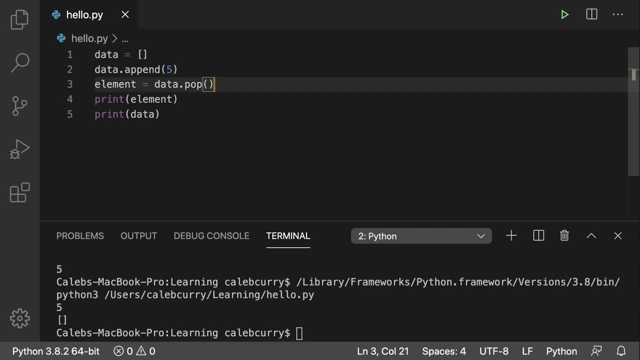 probably best just to stick to the basic operations of push and pop. Gosh, Claire, why do you always torment me? Now you may also want the peak operation, which is to look at the last element, and that's pretty easy. What we're going to do is we're just going to append that data. 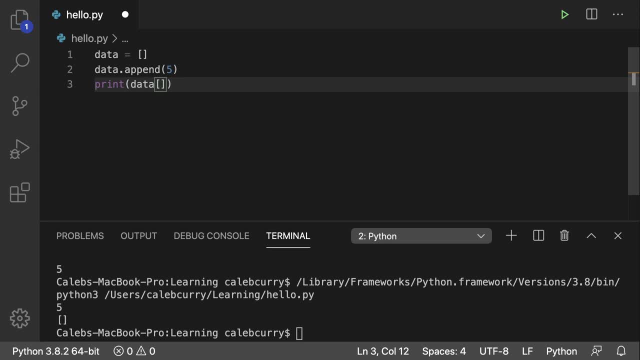 And what we're going to print is data and for the index just say the length of data And then subtract one. The length of data is always going to be one higher than the highest index To peak at the top of the stack. you just need to look at that last element. 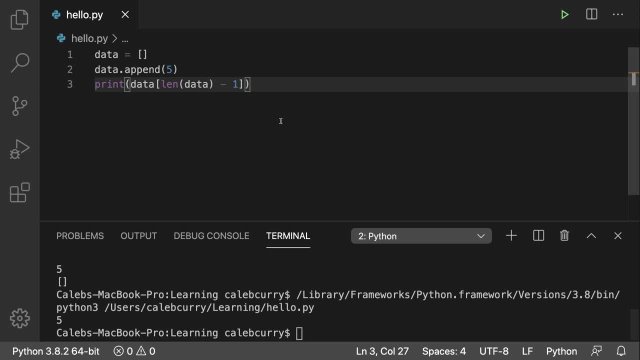 last element. So running this and we get five. but note that after this, if we print data, it's going to still have five inside of it. So we didn't actually pop that off of the stack, we just looked at it. Now, if you want to visualize a little bit more about how a stack works, it might help to do. 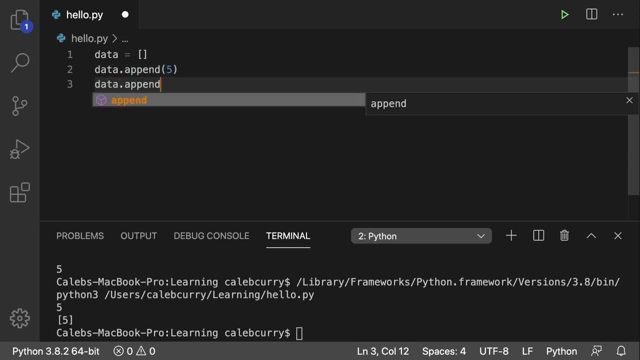 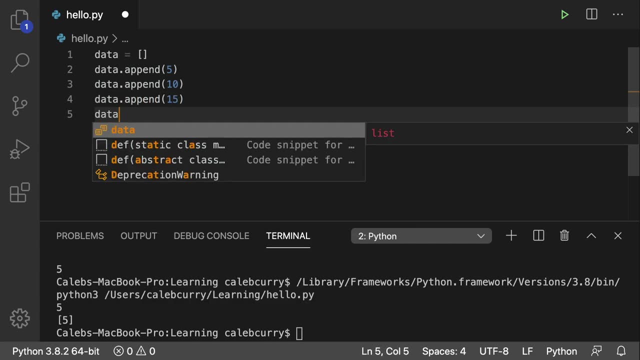 a couple of operations. So let's go ahead and say dataappend, and we'll do 10 and then dataappend and do 15, dataappend, 20 and then datapop, datapop. Can you predict what the list is going to look like when I say print data? Well, to understand how that works, we add five, and keep in mind that. 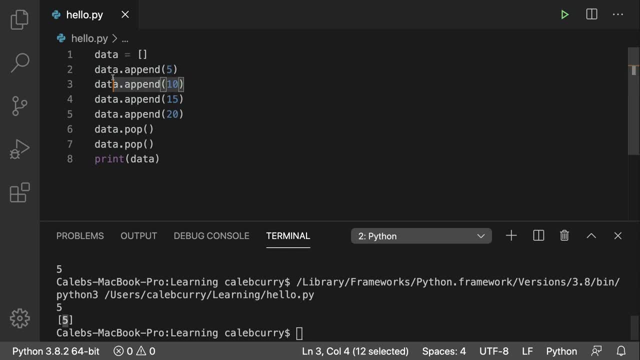 it's going to be the leftmost number. So when we append another number it's going to show up on the right of five. So we'll have five comma ten comma, fifteen comma, 20, and then, when we pop off the next two elements, we get first get rid of that 20, and then 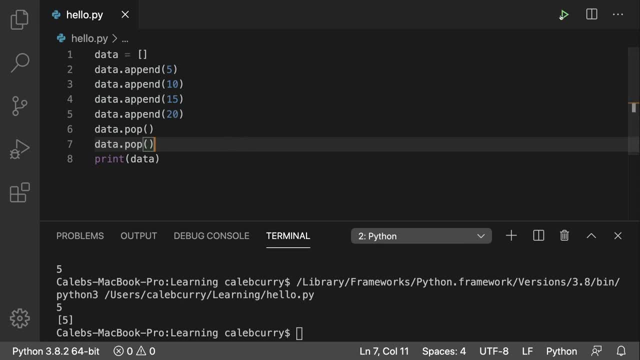 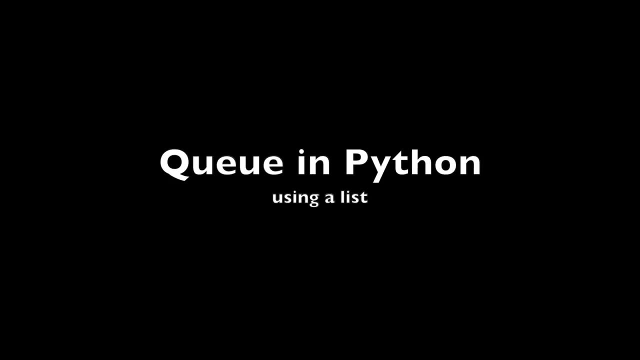 we get rid of that 15.. So we're left with just five comma ten. We run this and that's exactly what we get. So that is how a stack works. Now let's take a look at a queue. So the only difference. 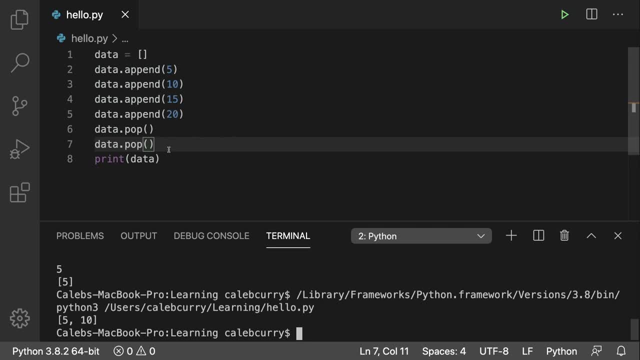 here. if you want to continue to use a list as the data structure of choice to implement a queue, the only difference here is that the list is going to be the list. So, if you want to continue to use a list as the data structure of choice to implement a queue, the only difference here is that the 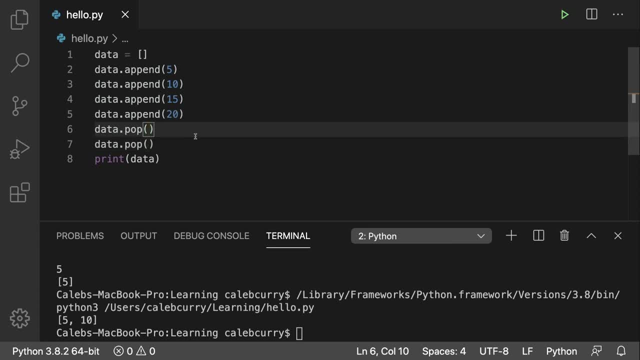 list is going to be the list. So if you want to continue to use a list instead of just using pop with no arguments, you're actually going to pass in a zero, And in this we're pretty much just considering the left of the list. So if you look down here at the bottom, the left is going to be the front. 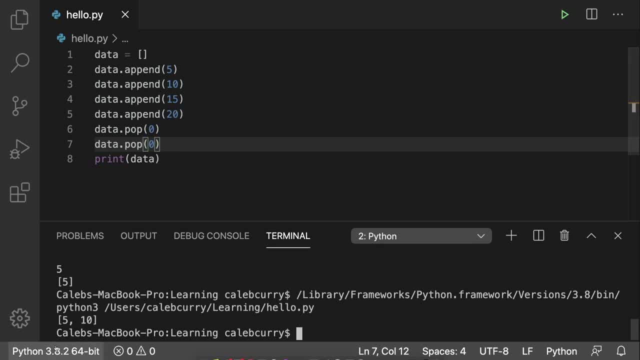 of the queue. So when we pop index zero, we're actually removing the leftmost element. So now, what this is going to do is it's going to add five, then behind it it's going to add ten, behind that it's going to add fifteen, and then behind that it's going to add twenty. When we pop 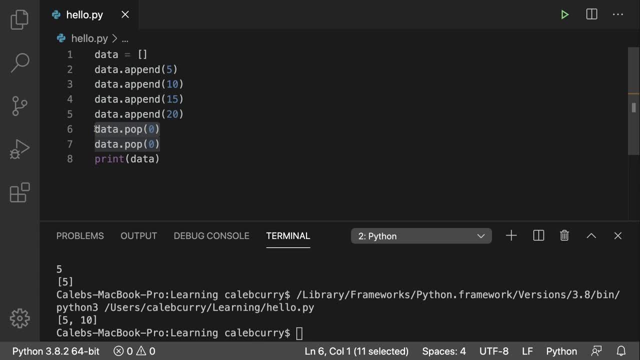 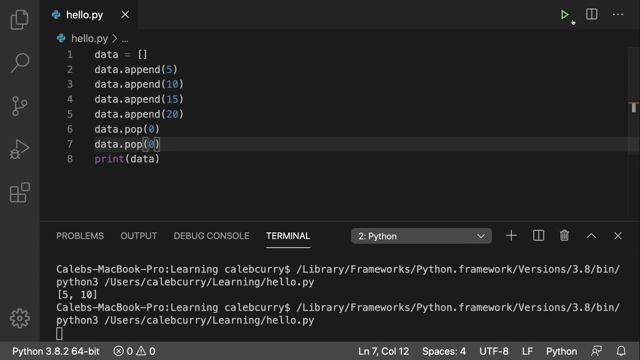 this first element. what it's going to do is it's going to remove five, and then this next pop is going to remove ten, So we should be left with fifteen comma twenty. We run this and that's exactly what we get, And, as always, this is returned. so if we wanted, we could assign it. 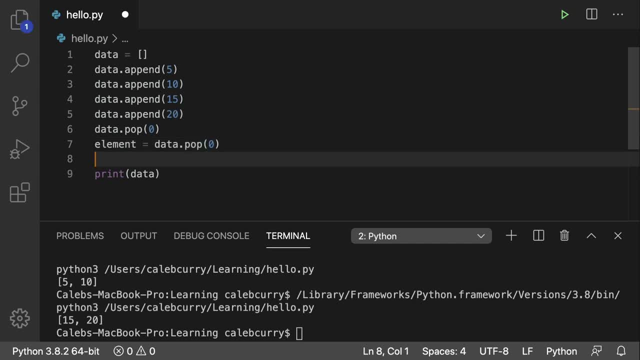 to a variable and then use it later on in our code. So, for example, we'll just print element and, running this, we get the value ten there. So that's the one that's popped right there. Now the naming here is a little bit different than what we're used to, So we're going to go ahead and 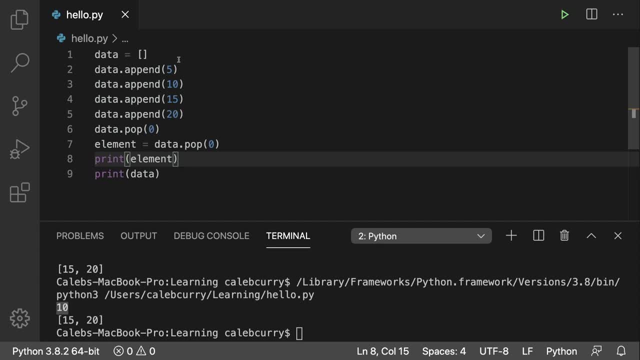 make it a little funky, But if you want to basically correlate these names to the operations for a queue abstract data type, the append is going to be the in queue and this pop down here is going to be the dequeue. If you want the ability to do the peak operation or to look at the element, that's. 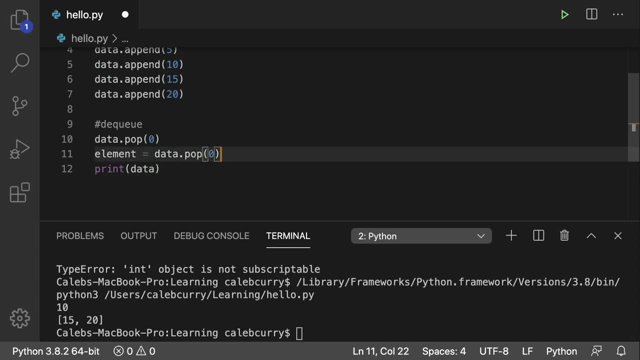 going to be dequeued. it's actually pretty simple. All you have to do is say data index zero and that's going to look at the leftmost element, in this case fifteen. So when we run this, we get the value fifteen, but that doesn't actually remove it from the queue. So that is how you would do it with a. 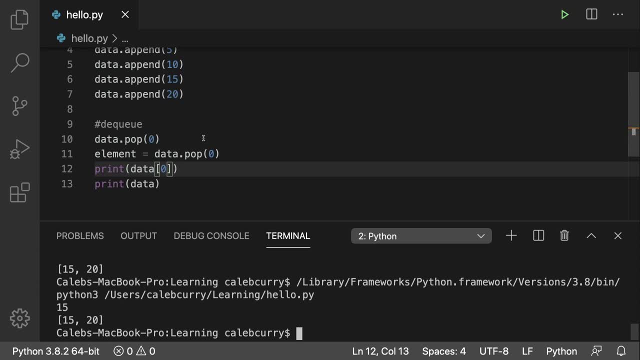 list. However, the downside here is that each time we pop an element, all of the other elements in the list have to be scooted over one index, which is a time-consuming operation if you were to have a pretty big list. Another way to think about it is: it's an operation that 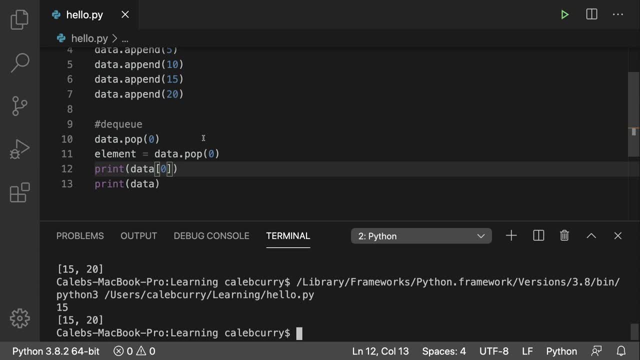 is O of N, So it's dependent on the list size- pretty much has to go through the entire list, moving all the elements over. We want to avoid that if possible. so there's actually another option we can use and that's going to require an import. So here's what we're going to do. 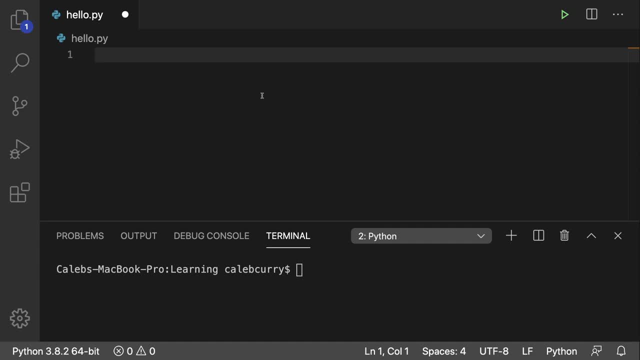 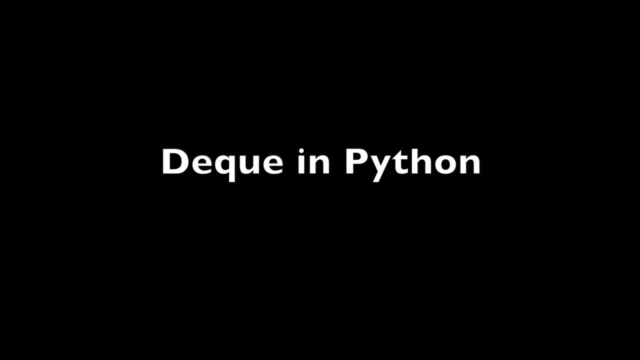 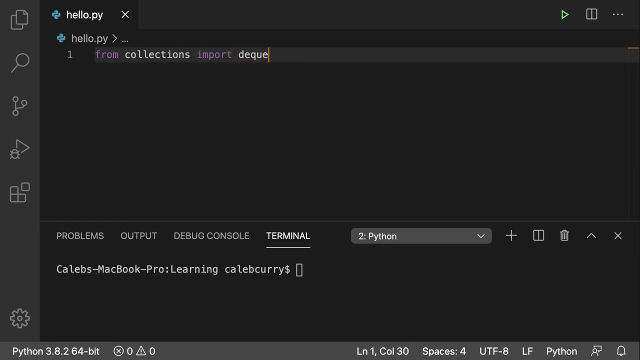 we're going to clear out our code, our terminal, and we're going to import a tool that we can use called a deque. So from collections, import deque. I called this a, a dequeue in the previous video, but whatever, I'm pretty sure it's pronounced deque. 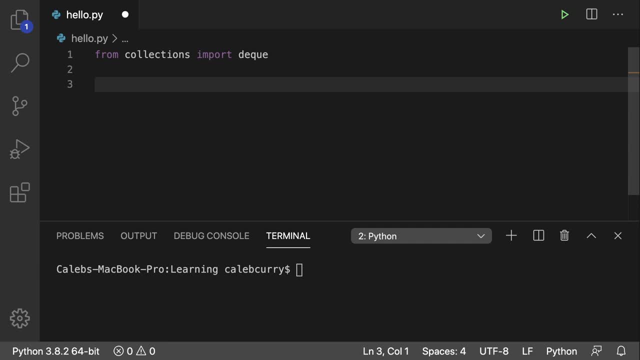 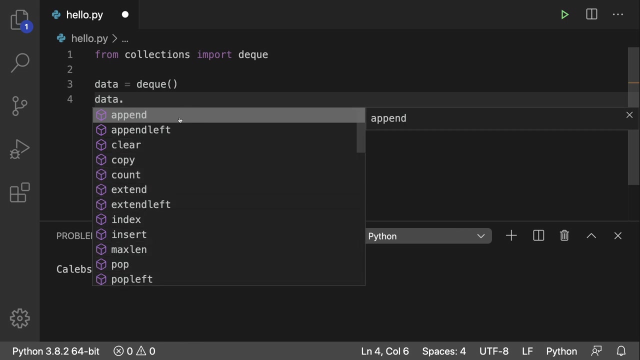 And to create a deque. what we can do is we can say data is a new deque, in parentheses, and the way you add data to this is pretty similar. You just say data, dot, and then here's all the operations we can use. So we'll say append. Let's use some strings this time, Caleb. 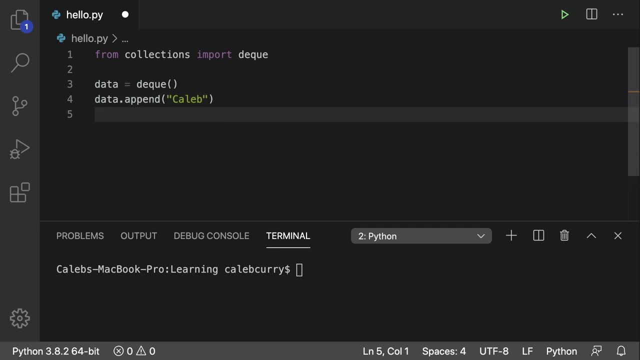 And then to remove this data. there is a special method on this So we can say data dot pop, but not just normal pop or a string. So we're going to make sure that doesn't stand out muy, we're actually going to pop left. 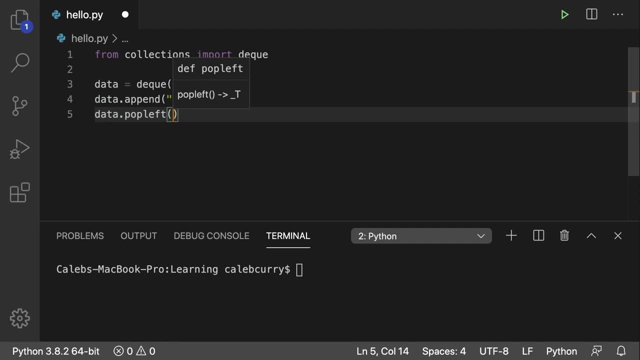 And this one doesn't require us to pass in zero, because it already knows we want to remove the leftmost element. So doing that should return the data. So we'll just say element and assign it that return. So then we should be able to, after this print element. 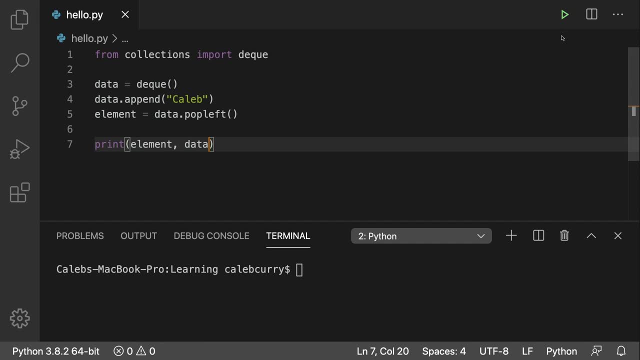 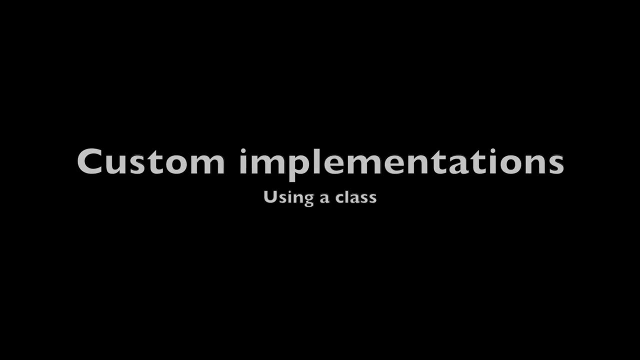 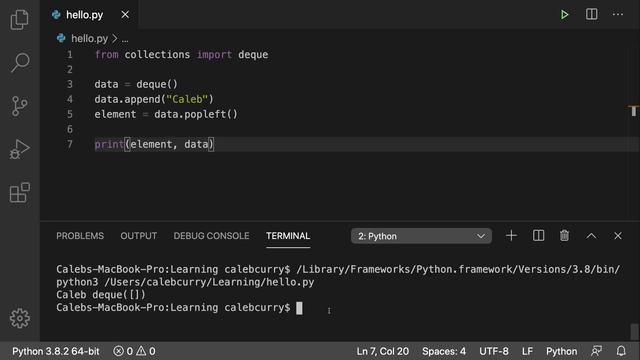 and we'll also print the list just to confirm that it's empty. So, running this and you can see we got Caleb and then we got a deck of zero elements. Now, if you ever need to be absolutely 100% strict with what operations can be used on a stack or queue, 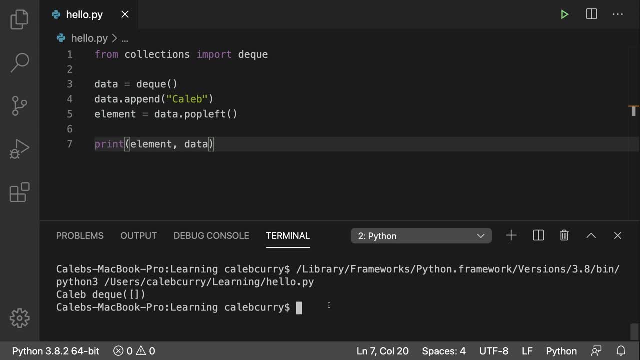 or pretty much any structure you're creating. you can create a custom class. So I'm not going to get super into this, but there might be a situation where you need to create a custom stack class or custom queue class or custom any class. 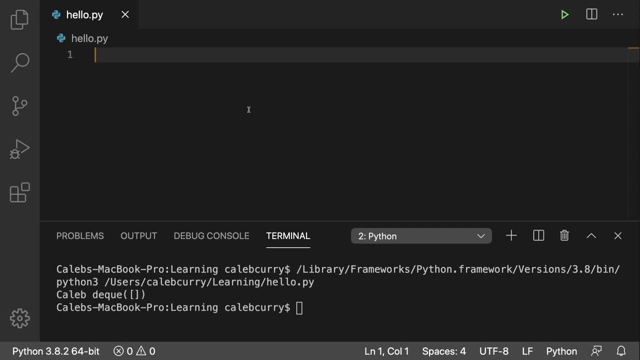 And if you're in class, the teacher's probably going to tell you to create all kinds of useless classes. So let's just go through an example of that, where we create a class called a stack And in here we're going to define an init method. 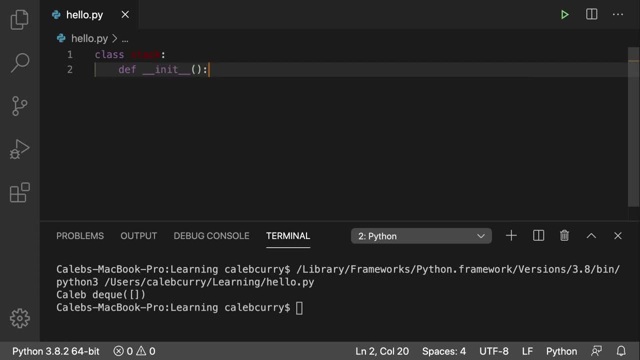 and this is the constructor. This is what is invoked when we create a new stack, And I'm actually gonna give this a capital S here. So the only parameter in here that you absolutely have to have is called self, which refers to the object that's being created. 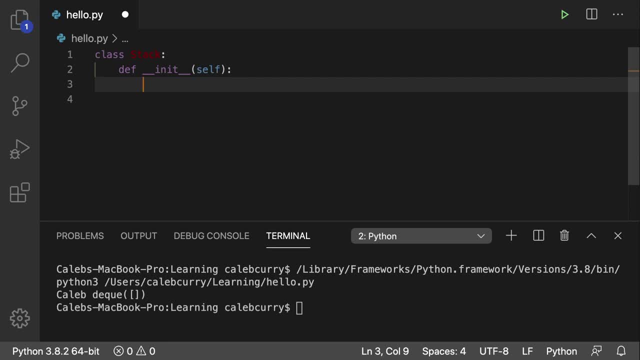 And then inside of this method you can define any attributes for the stack. So we'll just create a class, we'll just pretty much create a wrapper for a list. So to do that, we can say: selfdata is an empty list. 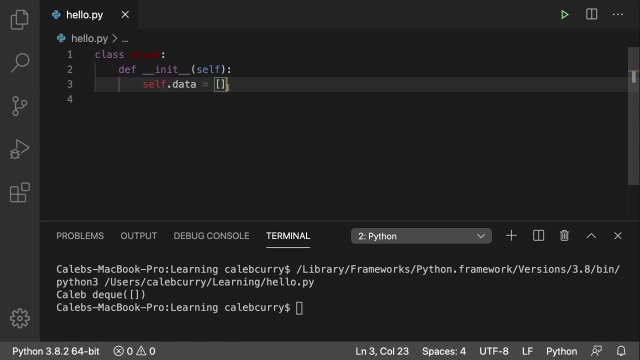 So it'll initialize it to an empty list. whenever we create a stack, We can also create methods for the stack. So, as an example, we could say def and we can name it appropriately to match the stack behavior. So we can call it push. 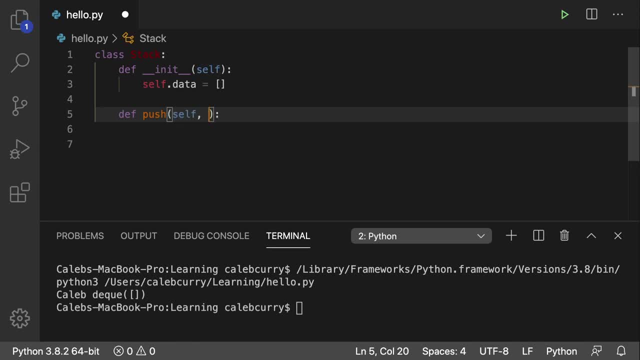 This is also going to require self, And, in addition to self, we're going to take the data to be pushed onto it, So we'll just call that data, And here's what we're going to do. We're going to say selfdata. 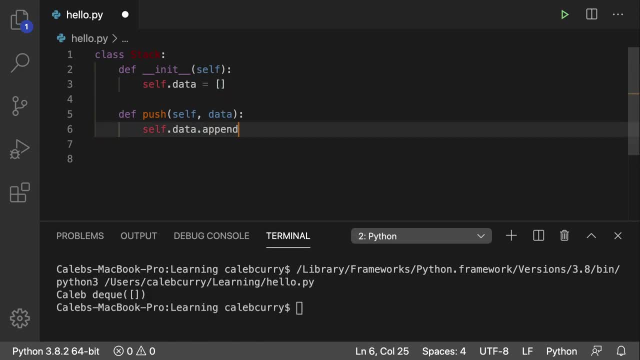 which refers to this list here. append and pass in the data parameter here. So you can probably tell we're not doing a whole lot. We're just pretty much giving a new name to something that already exists. but you could define any kind of custom logic in here. 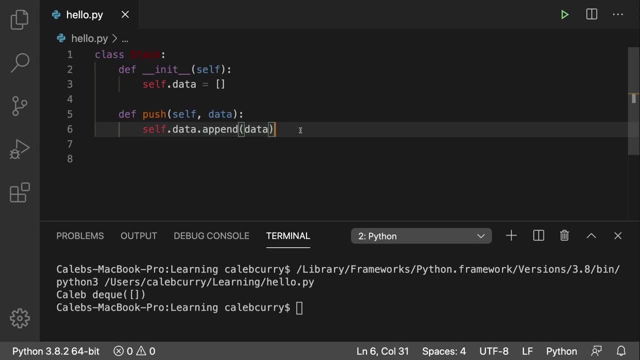 or force a certain behavior, whatever you need. We're also going to create a pop, So def pop. this is going to have self, but we don't need to pass in any other data. It's always going to remove from the same index. 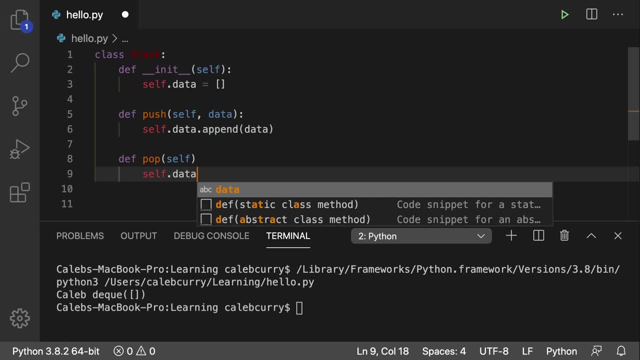 So we don't need to take that as an argument. Then all we have to do is say selfdatapop and return this. Now it's a convention inside of Python Whenever you have a private variable that is not really supposed to be exposed. 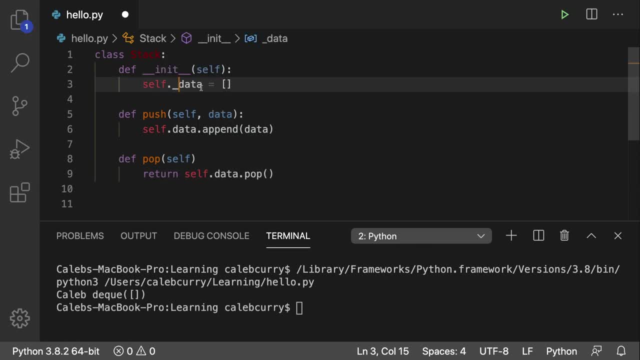 you can just prefix it with an underscore. So we'll put underscore data and update that throughout this code, And now we can practice using this. see if I got any errors anywhere. So what we're going to do is we're going to create. 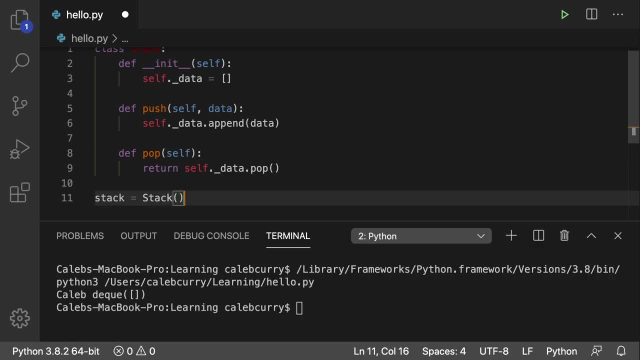 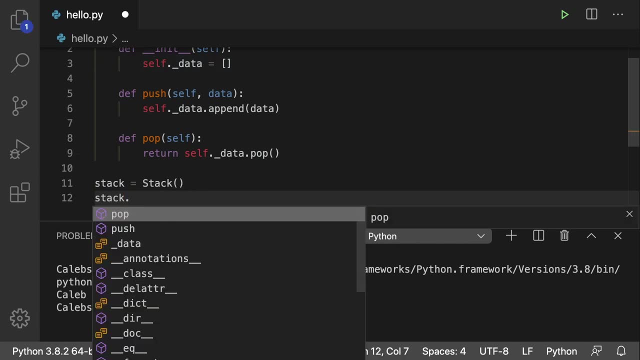 a new stack variable. So to do that, we just use the uppercase stack. That'll invoke this initializer here, And then we can say stack And look here, the only methods we have available to us now are pop and push, So we pretty much restricted, you know. 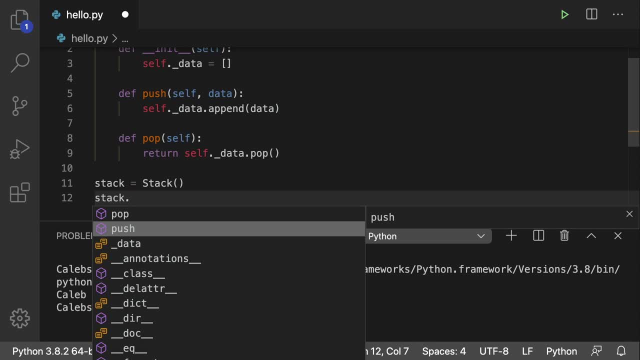 we've restricted just to pop and push. Now Python is fairly open, So if they really really really want to access that list, they can just by saying underscore data And then they have all of these methods. However, it is clear from my perspective. 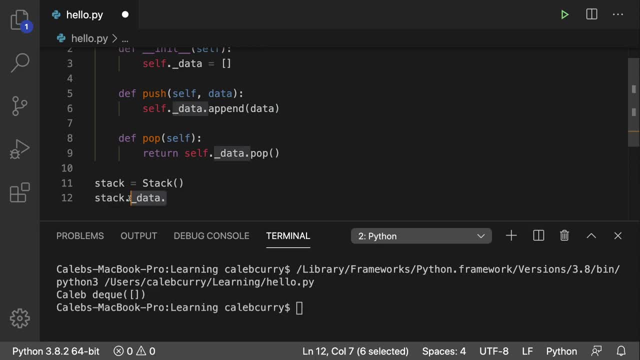 as the user of this class, that I'm not supposed to do that because there's an underscore here. I should just be using these methods here So we can, for example, push some data on and then we'll just get that data back out by saying stackpop. 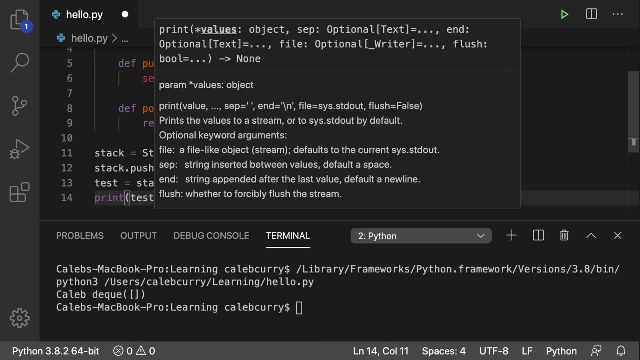 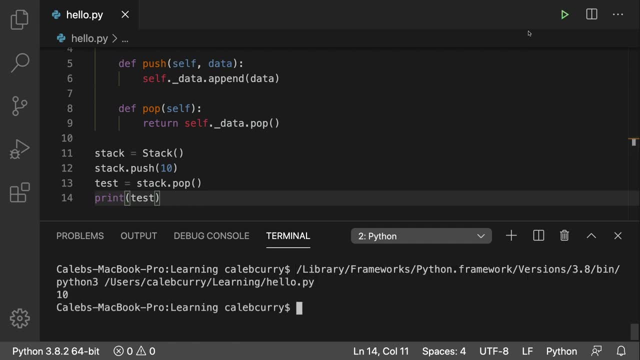 And then let's print test. So let's see if this works. I probably screwed something up. We'll run this. Oh hey, believe it or not, it actually worked. All right, so that is how we create a custom stack. 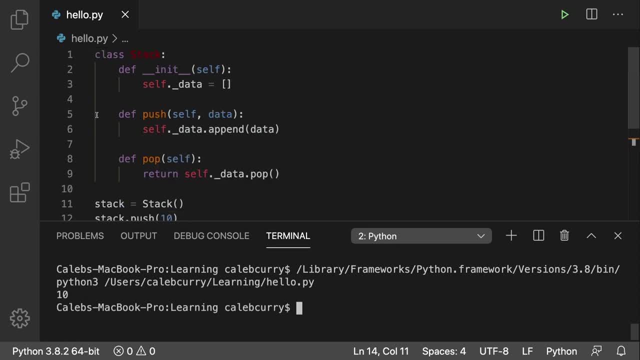 Now it might be silly, but the point here is that we can basically define particular things that need to be met, such as push and pop, And then the actual logic to do those can be anything. We could do a similar thing by creating a stack. 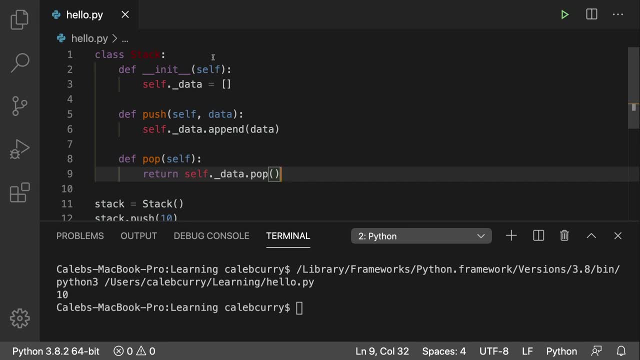 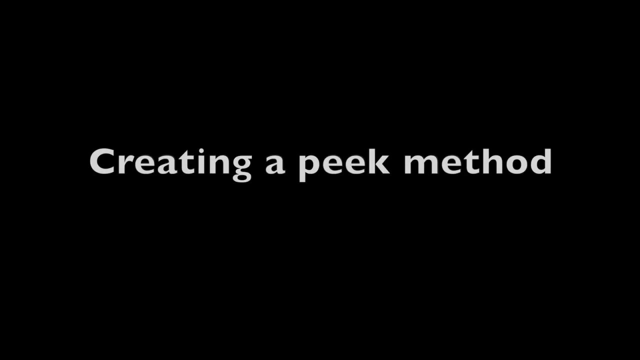 creating a class for a queue or a priority queue, a heap, a map, whatever abstract data type we're trying to represent. We can do that using custom classes, and the implementation is irrelevant. All that matters is how we use that class. Right now, this class is pretty simple. 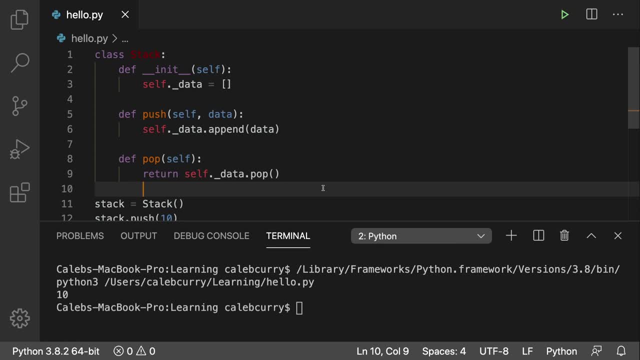 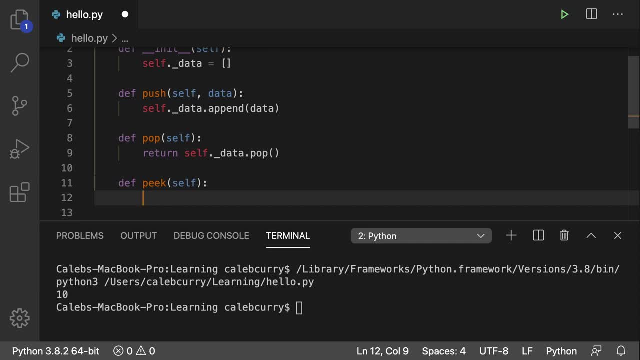 So, for example, we could create a method in here. So we could create a method in here, And for this all we would have to do is return self underscore data and then just get that last element, So we would get the length of the same structure. 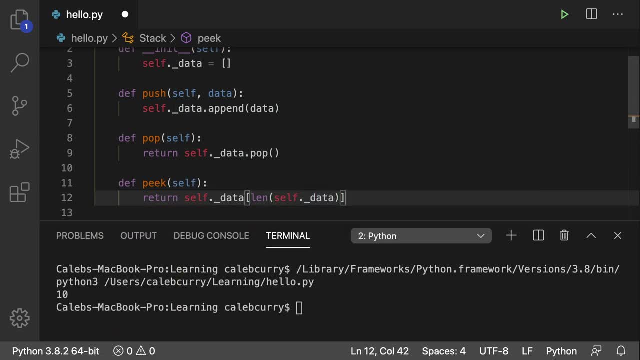 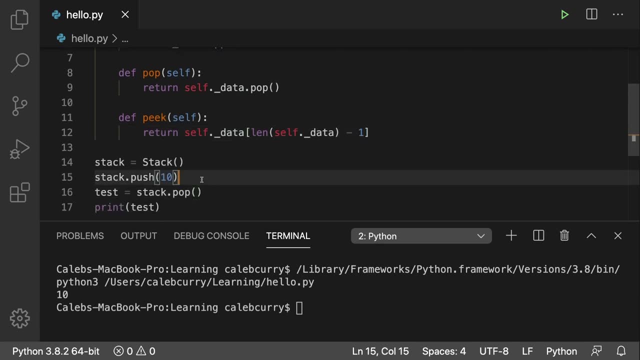 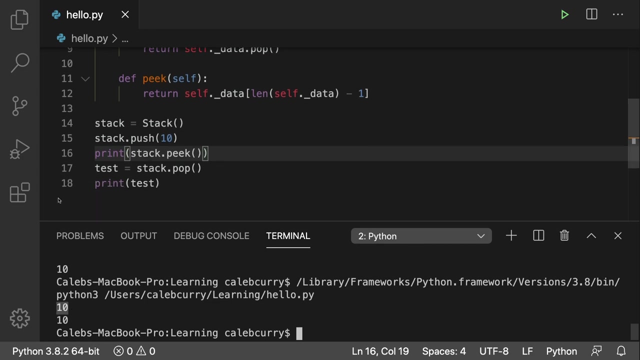 self dot underscore data and then, outside of the length, just subtract one. So let's try this out: before we actually do this, actually pop something. let's print stack dot, peak and we should get the value 10. and we do, we get the 10 for the peak and then we actually end up popping that data off, which is 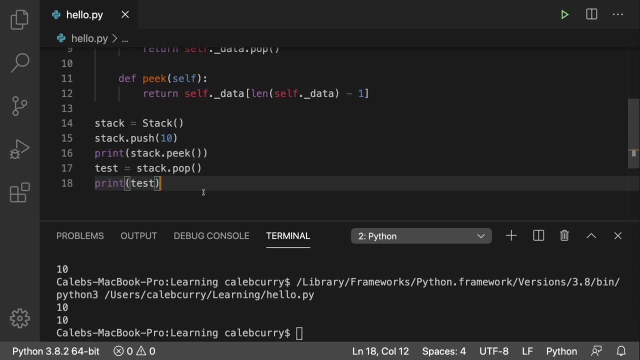 where that second 10 comes from when we print this variable here. so hopefully that lets you see some of the different capabilities we could do when it comes to creating our own custom classes. right now we're just using a stack, but you could create one for a queue, for a heap, a priority queue, a tree. 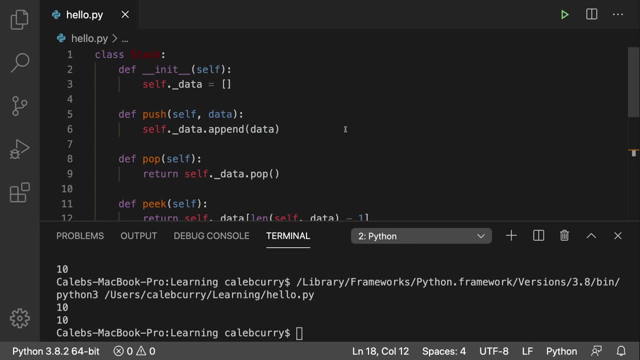 whatever structure you want. you can create a class to represent that. the class is going to define the different behaviors and different things that need to be stored and then when you actually go and create an object, like we did here, that's when you create an actual example of whatever we're working. 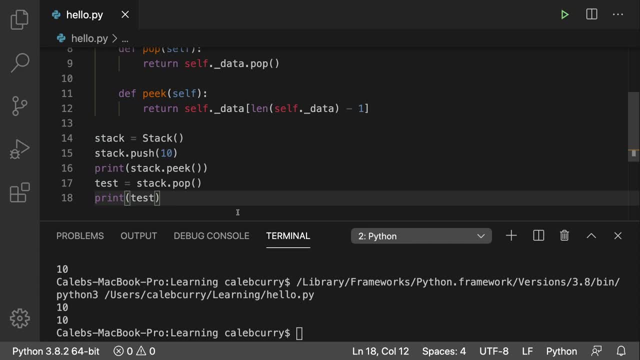 with. so we're creating an actual stack and using it in these lines of code. so hopefully that was helpful. i'm sure you could take this code and adapt it for other programming languages and we'll see you in the next video, and in fact it'd probably be a good practice to try it in a few programming languages to get some. 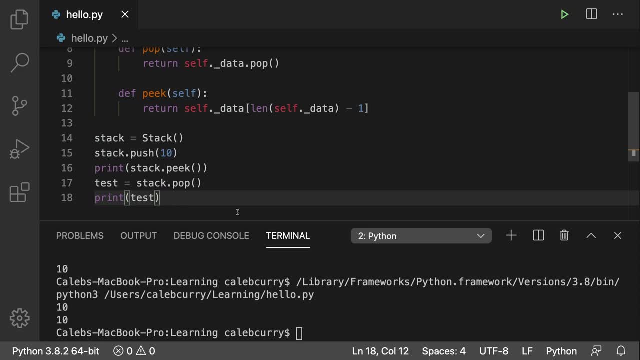 experience. that's one of those things where, like, i'm not actually going to do it myself because i don't really want to, so i'm just going to move on to the next video and hopefully you guys are excited. let me know if you enjoy these hands-on videos or if you prefer the conceptual videos. 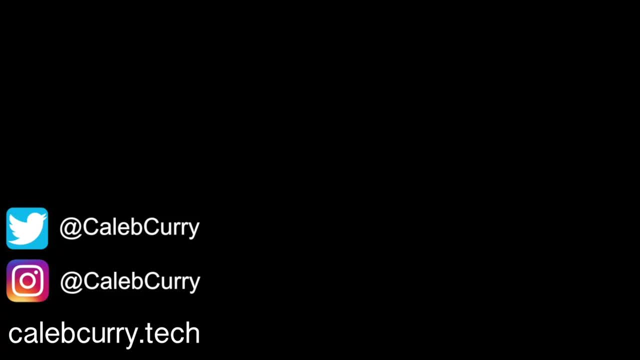 in person. stay tuned and i'll see you in the next one. bye.